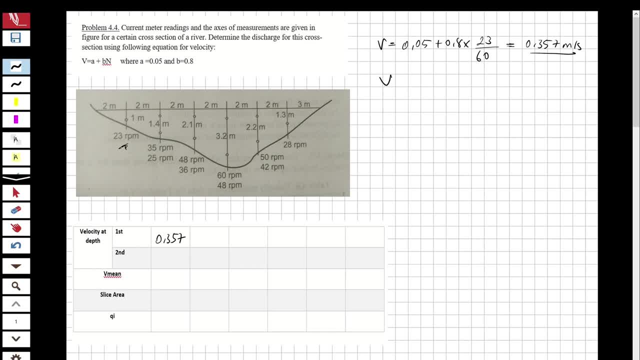 let's do it for this one: 0.05 plus 0.8, multiplied 35 over 60.. And this will be equal to 0.516.. 0.07.. And for this one, 0.05 multiplied 0.8. Sorry, not multiply. it's going to be plus, it's going to be summation. 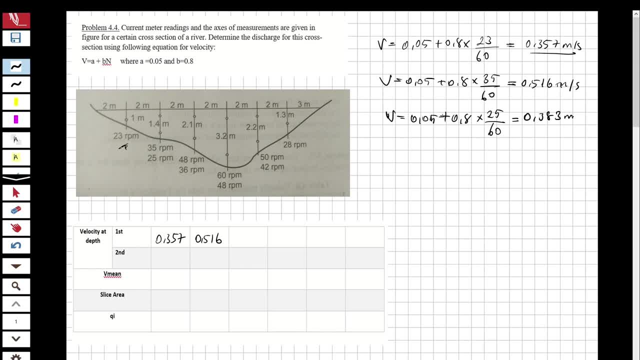 satisfied 25 over 60. And we're going to obtain all point 383 meter per second. I Think I don't need to write this all because now you can see How it's going to be. so I'm going to write just the velocities and we're going to try to solve the question. 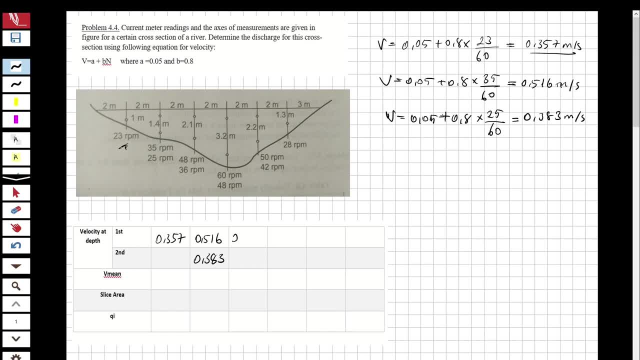 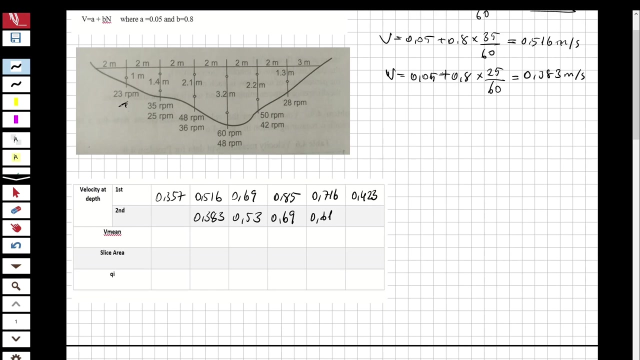 Okay, so I'm going to write here faster And For this one we are going to take the mean value of the velocity. Okay, mean value of the velocity. So this is going to be all point three, five, seven and the mean value of this. both will be all point four, four, nine, five and. 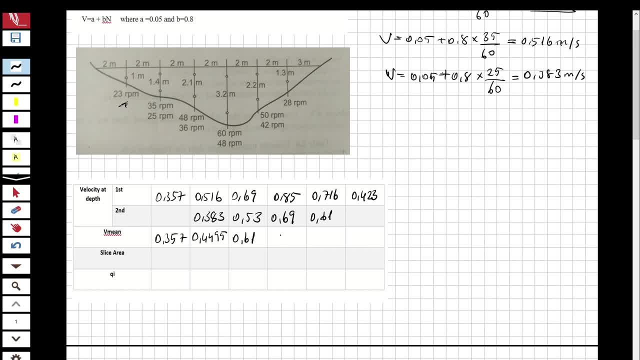 the mean value of this all point sixty one and this one all point seventy seven, and This one will be all point six, six, three, and this one will all point four, three, two or three. The main value means that I'm going to write here. Maybe someone 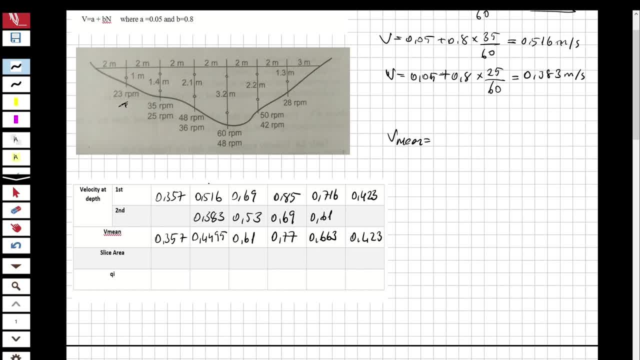 May confuse. For example, for this one, Okay, this is going to For one, this is two, There's a three, This is four, This is five and this is six. So for the second one, I'm going to do it All: point five, sixteen plus all point three, eight, three. 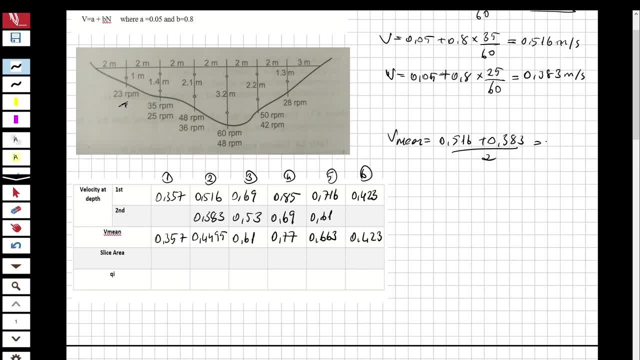 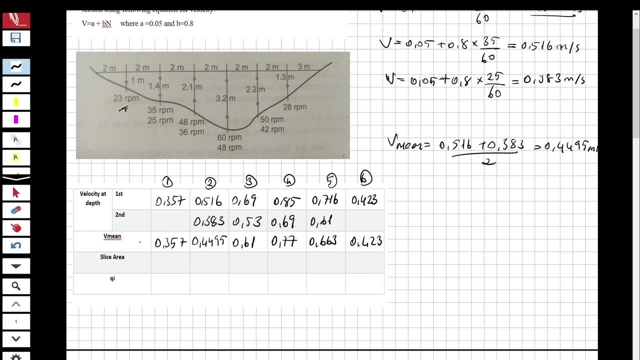 Do, I do two, and It's going to be all point. four, four, nine, five meter per second. okay, now we understand how we are going to take the Mean velocity. So now you know. the result has become like some fragment here, For now we are going to. 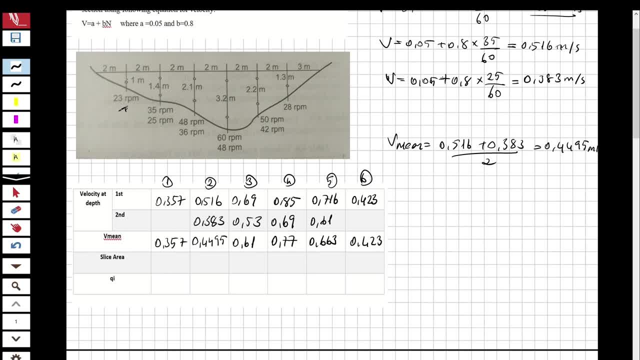 Calculate the slice area. ok, slice area, how we are going to be calcuate by doing two. divided this stream into slices. for example, From here to here it's going to be divided to: This is one meter, This is one meter and this is zero. We don't use it and 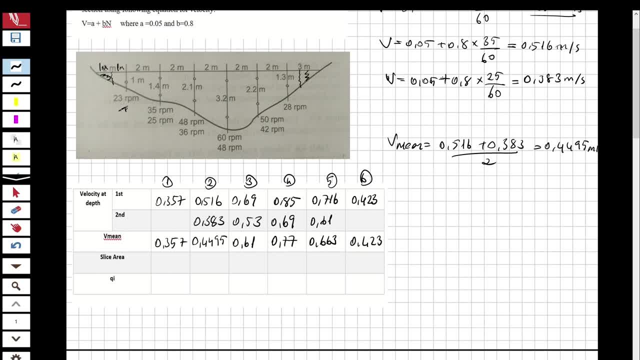 Also, this side is going to be divided to. this is going to be: uh, we don't use it as zero, okay, it's 1.5, this is 1.5, and going to take the all half of this sections. okay, and this one be one meter, this one be one meter, this one will be. 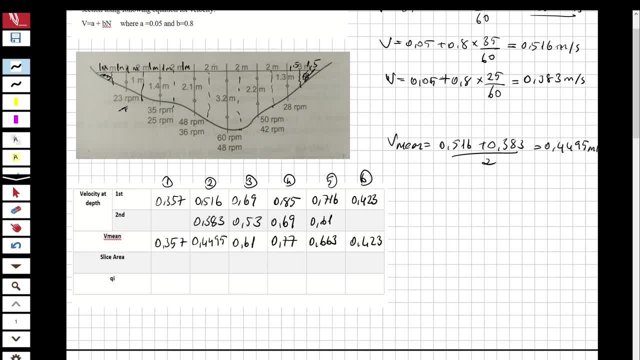 one meter, one meter, and this one, one meter, this one, one meter, one meter, one meter and one meter and also one. so now this, uh, i'm going to give and give them number. these numbers actually are for them: one, two. this is going to be an area. okay, now i'm gonna- sorry, no, not this one. 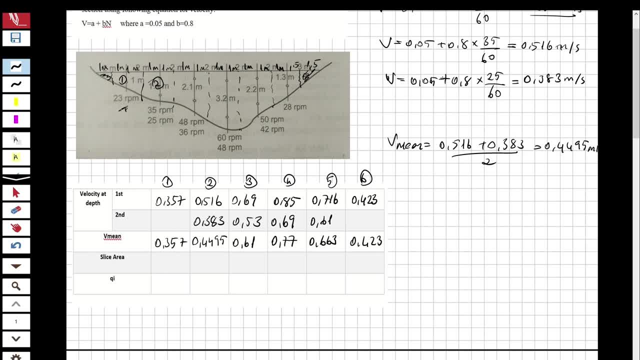 yeah, for example, from that that line until that dash line is going to be three. okay, the area of three. now this one, okay, this one will be area of three and this one will be four. from this dash line to this dash line. i can show- oh sorry, i can show you here this- between these two dash lines going to be: 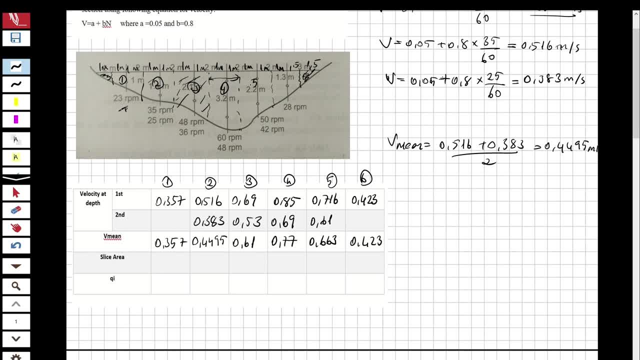 area four and this will be five and this will be six. okay, so now let's calculate the dashed area. what is this length from that point until that point? for example, for the first one, one meter, one minute, two meter. what is the depth? is one meter. two multiplied one is going to be two, okay, so, uh, let's calculate for the second part. 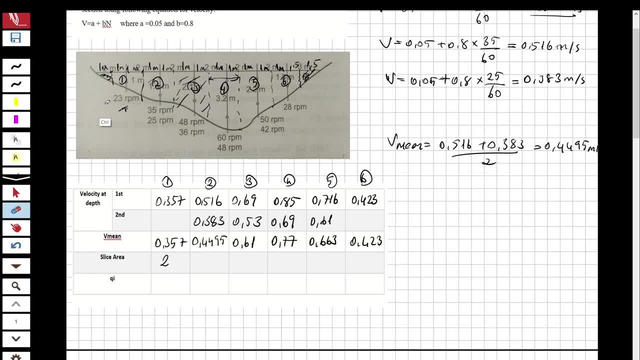 yeah, but now we can't see. actually, now you can see, but i don't know. now i'm gonna write from here. but one second. i did a mistake, sorry. yeah, now it is okay. so this is the second part. this is the third part. this is the fourth part. 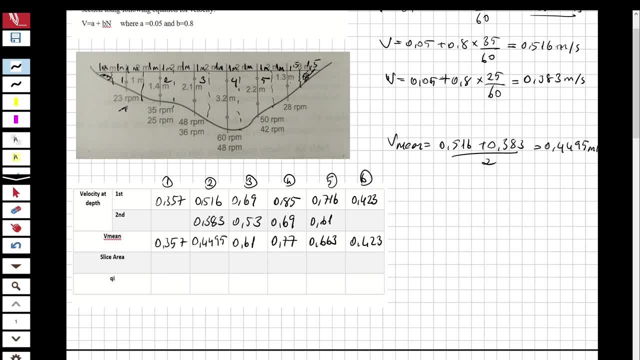 this is the fifth part and this is the sixth. so this is the sixth part, okay. so, uh, from that point, we actually we made it for the first part, but we are going to do it again- okay, so for this one, from that point until that point, it's two meter. right, we have multiplied this length, also the depth. 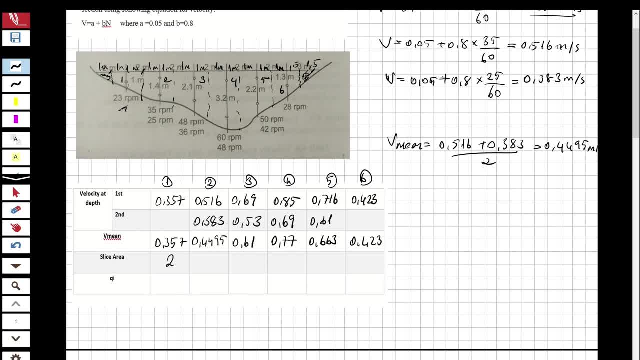 so it's going to be. the slice area will be two. let's go to. for the second, this is going to be one, one, two multiplied 1.4, it's going to be 2.8. and for the third part, it's going to be one meter, and one meter because it comes from this half. 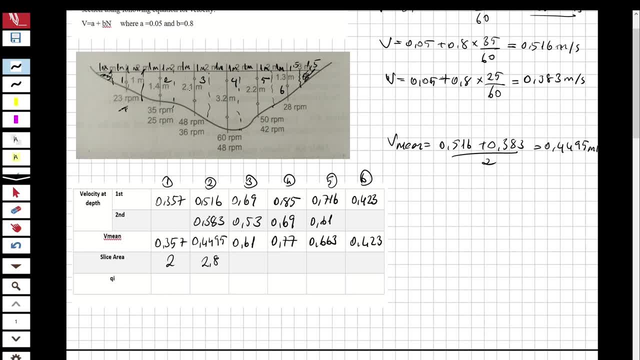 and this comes from this half. so one, one, two multiplied two point one, it's going to be four point two meter. okay, and also for the fourth part, one meter from this part and one meter also from this part. two meter multiplied three point two, six point four. and let's calculate for the fifth part. 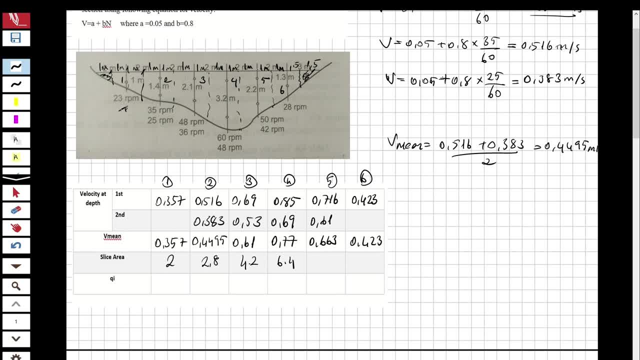 one meter from here, one meter from here, two multiplied 2.2, it's going to be 4.4. and for the last part, it's going to be a one meter from that part, because this is the whole, for example, this is the whole two meter, and i'm going to take the 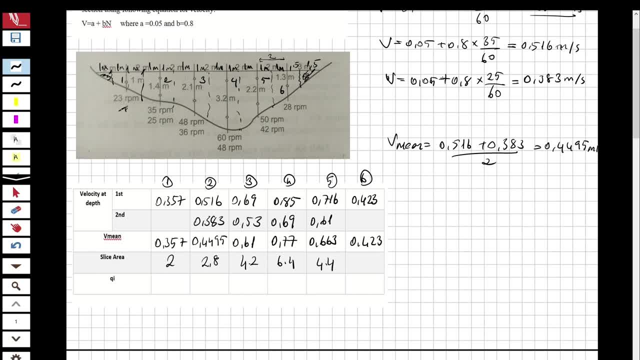 half of this to here. so it's going to be one meter and this is three, and i'm going to take the half of this to here. it's going to 1.5. 1 plus 1.5, 2.5 multiplied 1.3, it's going to be 3.25. okay, 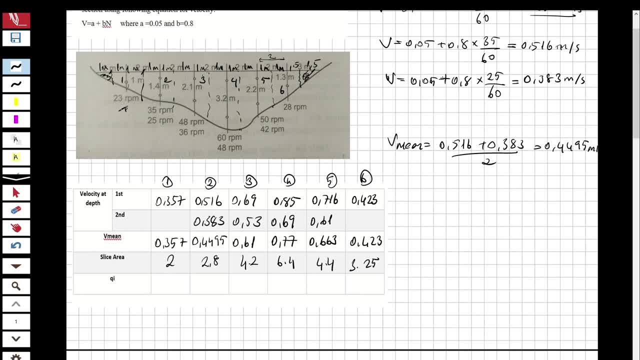 for this one. don't confuse. maybe this can be three. so you're going to. you're going to take 1.5. here it's going to be 3.25, 1.5. here you got it. so don't get confused. just try to understand how the 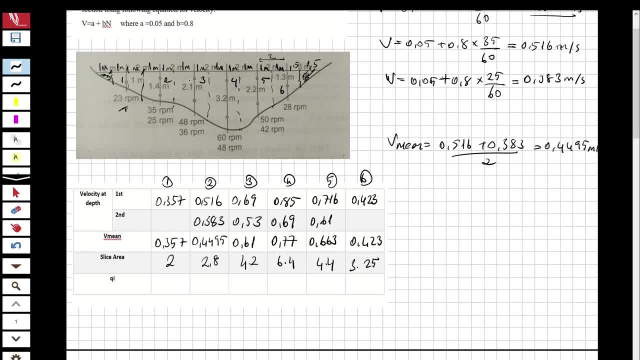 question is solved. the question can be shown as different, but the, the logic is the same. you got it, the logic is the same. so let's write the, the Q, the discharge discharge will be meter cubic over second. okay, but what is the discharge? this charge is we velocity multiply the area. okay, this is the. 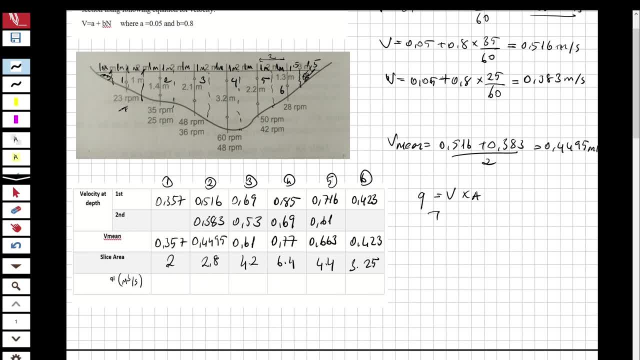 discharge. we are going to calculate one by one, two. you are going to take the velocity mean velocity, 0.357 x 2, 0.714. okay, and for this one, we are going to multiply it mean velocity, multiply the slice area, and we are going to obtain. 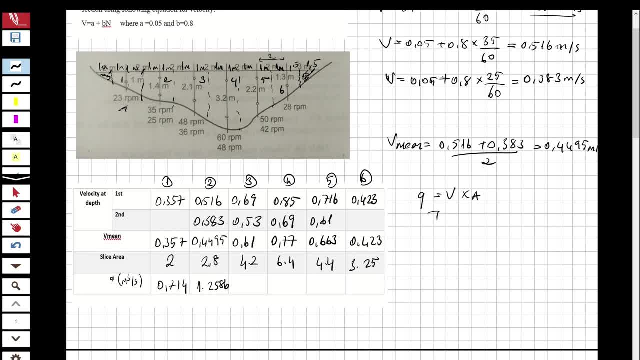 1.2, five, eight, six. okay, for this one, four point two multiplied all point sixty one, and it's going to be equal to two point five, six, two, and for this one, six point four, multiplied all point seven, seven, and we are going to obtain four point. 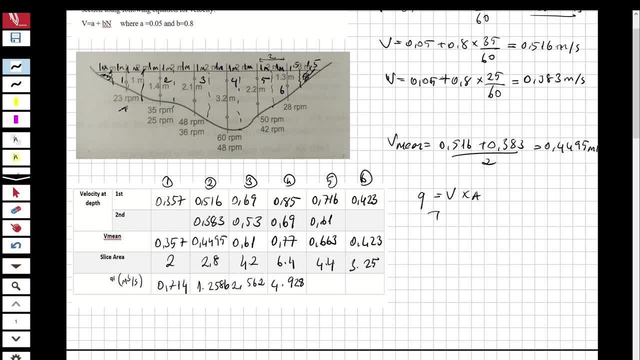 nine, twenty eight, and this will be four point four multiplied all, point six, six, three. this will be equal to two, 2.9172, and 3.5 multiplied 0.423. yeah right, 1.374. okay, now we are going to. sorry, we calculated all. 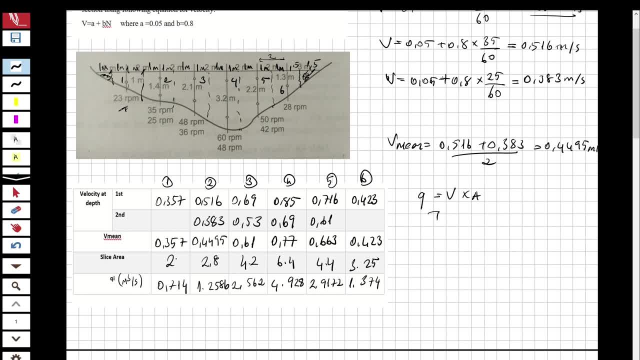 the discharges for the all cross sections. so let's determine the total discharge. we calculate all discharges now for the all cross section. the total discharge will be the summation of these six discharges. okay, there's six discharges: one, two, three, four, five, six. when we take the